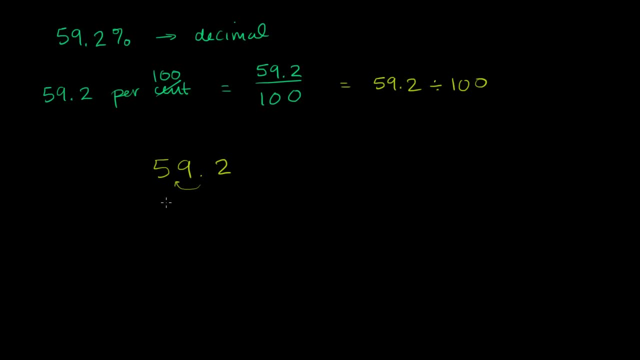 we would move the decimal over to the left once, We would get 5.92, but we want to divide it by 100, so we move the decimal over to the left again. We're dividing by 10 once, and then we're dividing by 10 again. 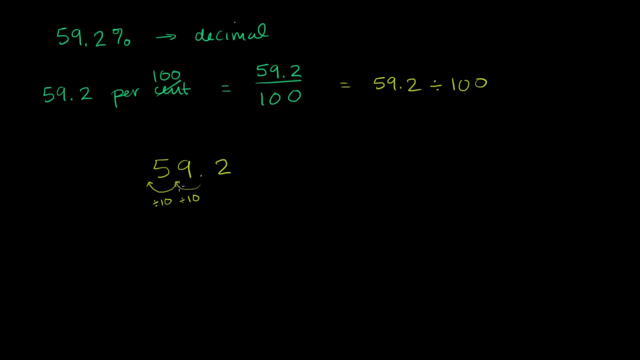 Divide by 10 twice, you're essentially dividing by 100.. So you move the decimal to the left twice, you get .592, and we'll just put a zero out here just to clarify things. and we're done. We've written 59.2% as a decimal. 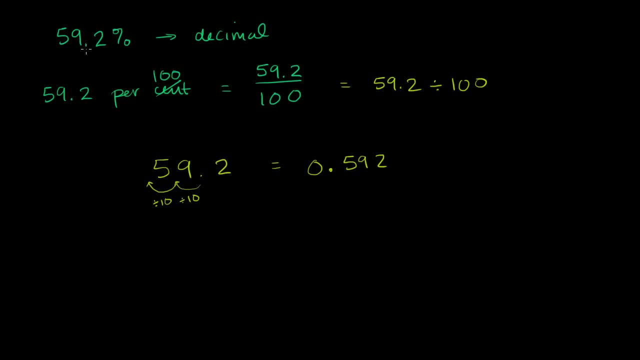 We essentially just divided this by 100, which is dividing by 10, twice moving the decimal once to the left and then another time. Or, since we're dividing by 100, moving the decimal twice to the left, and we get 0.592.